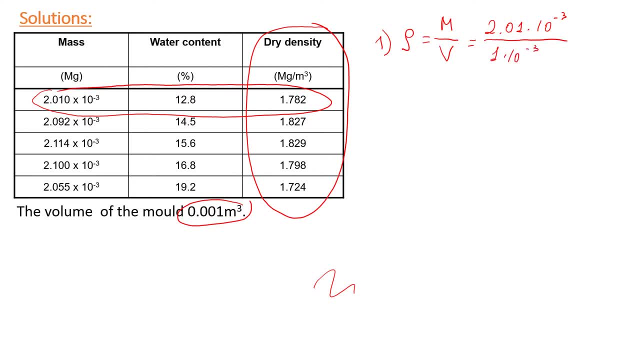 So it's 1 times 10 to the power of negative 3.. I change it to cubic meters and that will give us 2.01.. And the units will be mega grams per cubic meters. So that's the first step. The second step is we need to get the dry density. 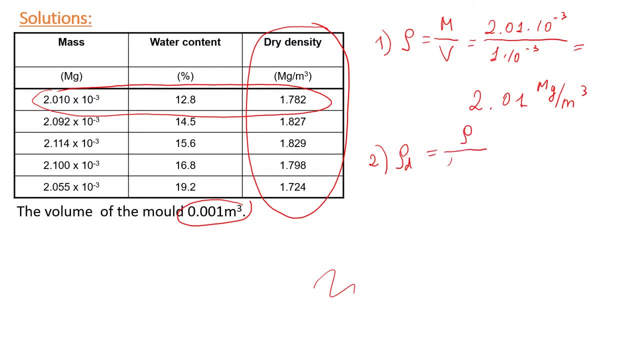 Dry density is bulk density divided by 1 plus water content. Again, for the first test, we'll have that the density is 2.01 divided by 1 plus water content. In this case we use the ratio for the water content. 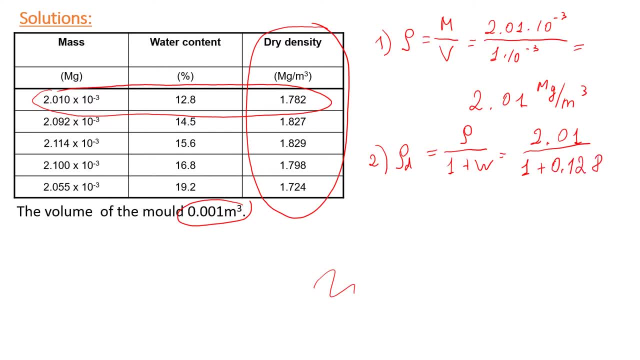 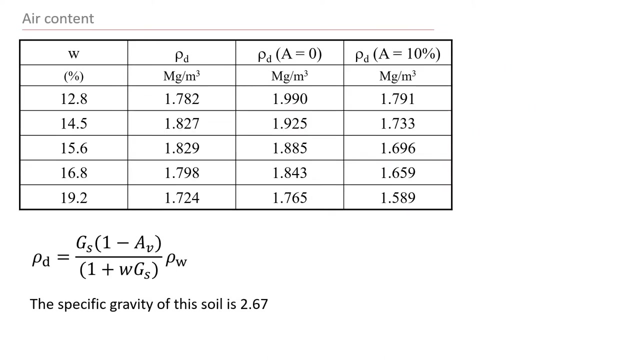 It's going to be 0.125.. And then we'll give us approximately 1.782 mega grams per cubic meters. So that's what we have here. in the first row, We repeat the procedure and we get dry density for each of the tests. 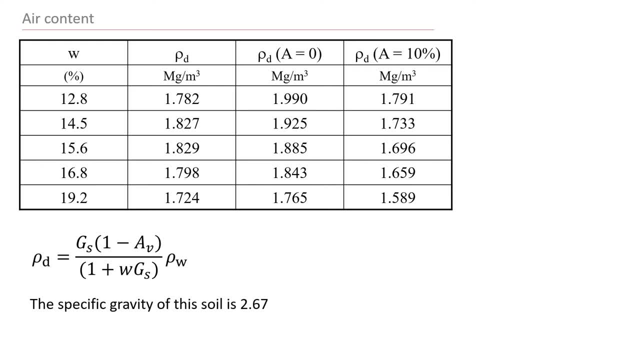 The next point is: let's see what is going to be the dry density If we assume that the air content is 0. And then we can do the same thing. For example, if we assume that air content is 10%, we can calculate the density for each of the water content that is given here in this table. 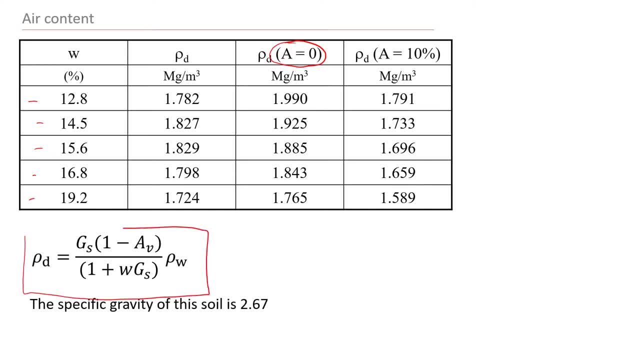 So to do that, we will use the formula which is given here And, for example, if we're thinking about water content and air content, it's 0.. So in this case, we're going to replace this parameter, a v, with 0. 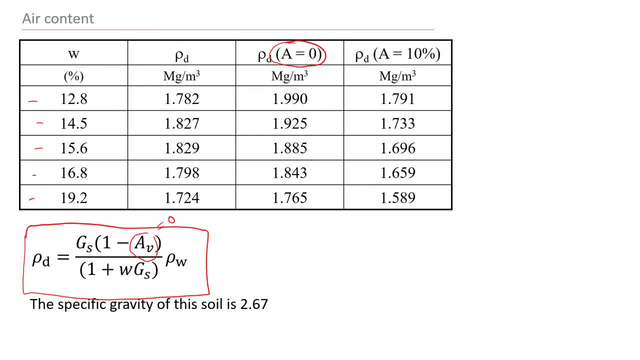 And then we'll calculate the dry density for this particular water content. So let's do it together. So dry density will be specific. gravity was given to us 2.67 times 1 minus. So for the first for this row, 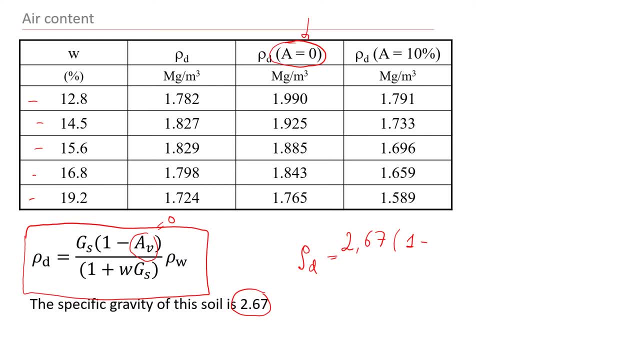 when we have 0 air content, we assume it's 0. Then it's going to be 1 plus water contents. It will be this one. So we're going to write 0.128 times specific gravity: 2.67.. 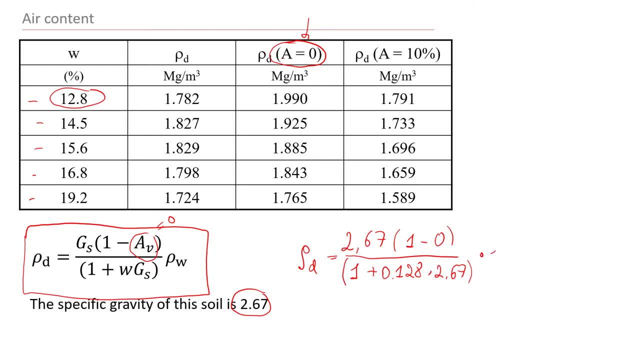 And then multiply by the density of water, Which is 1 megagrams per cubic meters, And that should give us about 1.99 megagrams per cubic meters. So this is the value that we have here in the first row. So we can keep doing this. 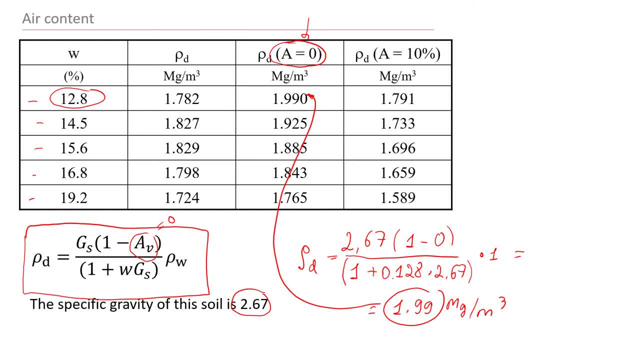 We use the same procedure. The only thing that we change for this column is the water content. So we change water content This way, For example, if we would like to draw a line where we know that air content is 10%. So in this case we're going to do the same thing. 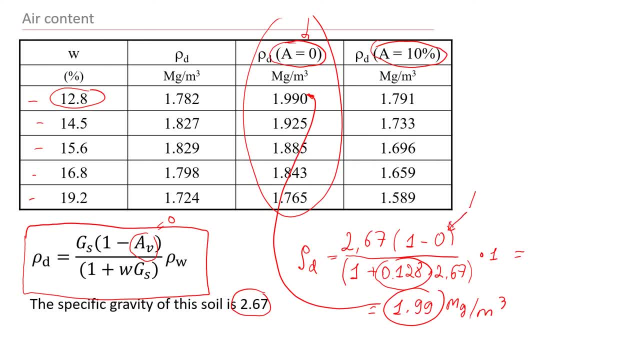 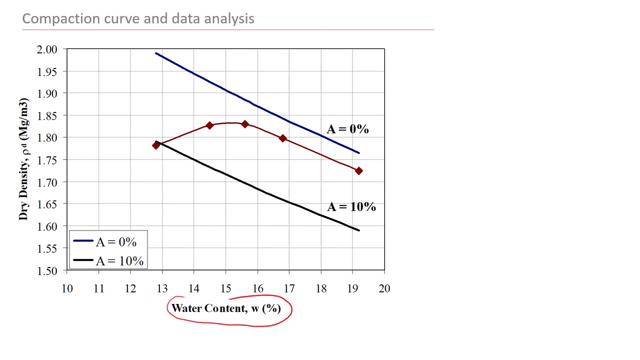 With the exception that here, where we have a v, we're going to write 0.1.. Remember to use the ratio, not the percentage. So these are the 10 results that we draw as water content Versus dry density. You can do it by hand. 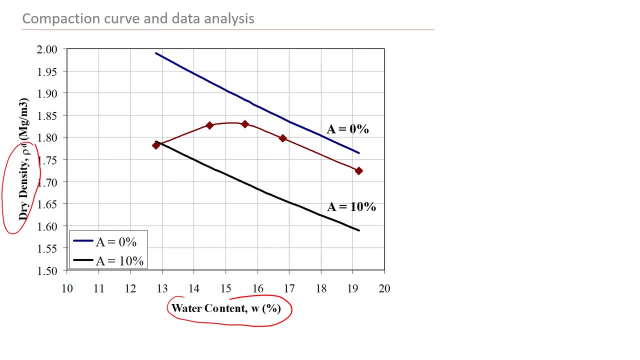 Or, if you would like, you can actually draw it using Excel. It is up to you. So what we need to do is we need to get the peak, And the peak will be somewhere here. That's the point. So this will give us maximum dry density. 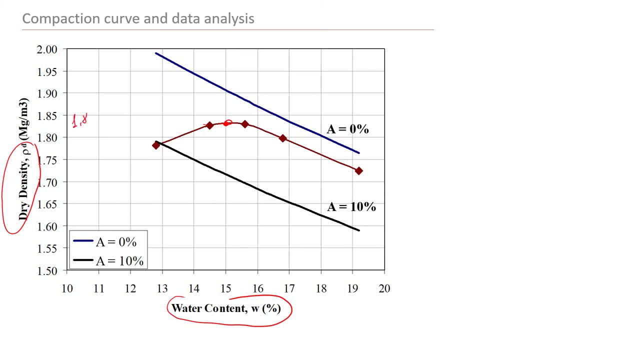 Which is about 1.83. Megagrams per cubic meters. So I'm talking about this point And it also gives us some what we call optimum water content, About 15.2%. So these are two major parameters that we get from this test. 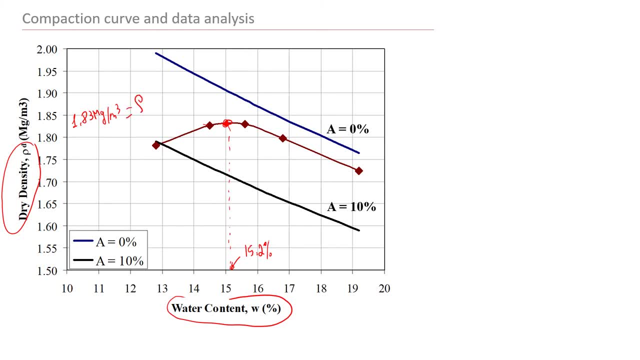 It's the maximum dry density And I'm going to write it here: Max. And this is optimum water content And this is the maximum air content. So these are the curves where we have air content 10%. So this curve will cross our experimental curve. 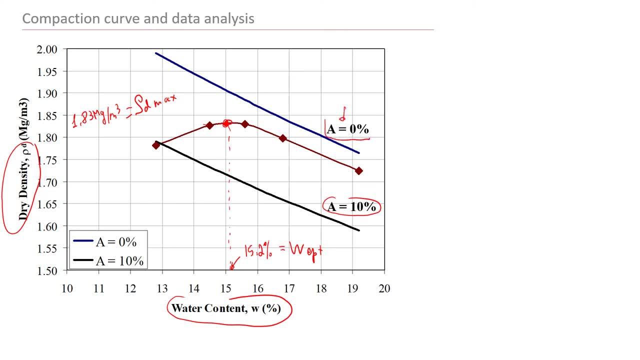 And we have this line where we assume that there is no air in the soil. It's not possible to achieve in nature, in real life. So this is a theoretical curve And this curve will never cross the experimental curve, This one. You see how, in this case, they never touch each other. 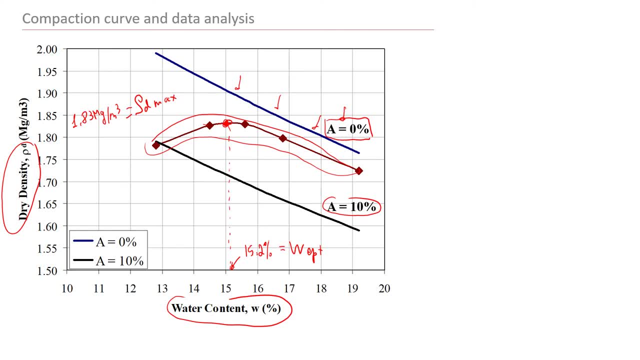 Another thing that you need to remember that in real life, in the field, It's very difficult to obtain this maximum dry density when we compact soil. That's why we would go for about 95%, Which is acceptable. So in this case we would calculate 95% of the acceptable maximum dry density. 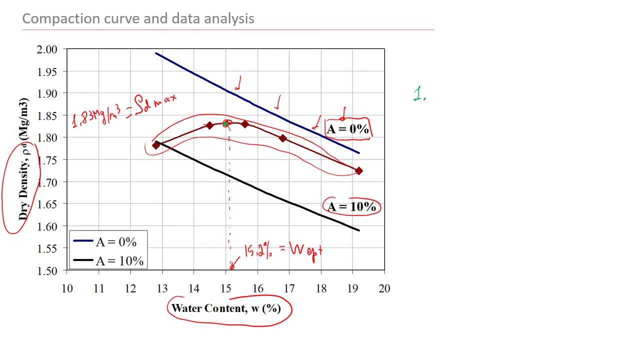 It will be maximum dry density: 1.83.. And 95% we just multiply by 0.95. It will give us approximately 1.74 megagrams per cubic meters, So 1.74.. I think it should be somewhere here. 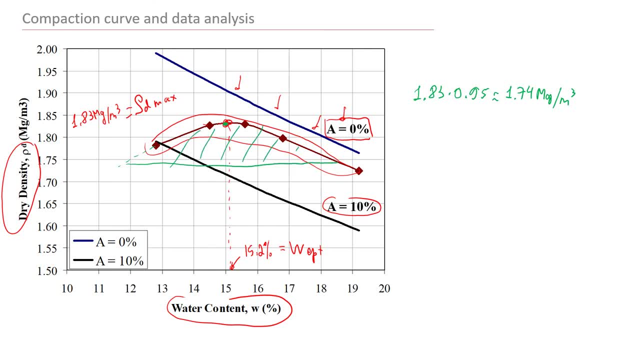 So this range of maximum dry density Will be acceptable in the field If you do a test in the field And if you notice that the maximum dry density of that compacted soil is out of this range. So it's below the maximum dry density multiplied by 0.95.. 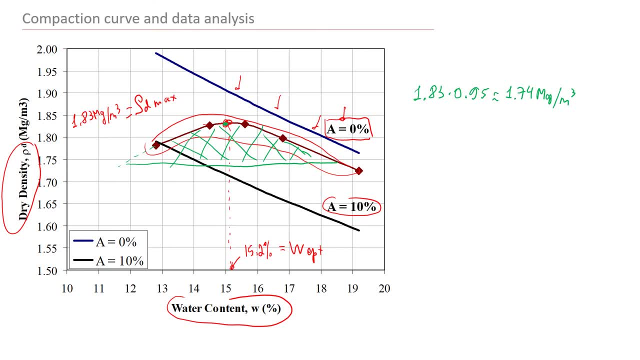 In this case, the compaction process needs to be redone With the water content. The assumption is that the water content in the field Should be close to its optimum water content Plus minus 1.5%. And the final point of this exercise.